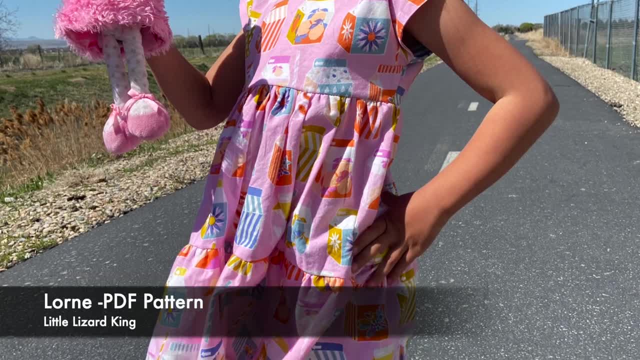 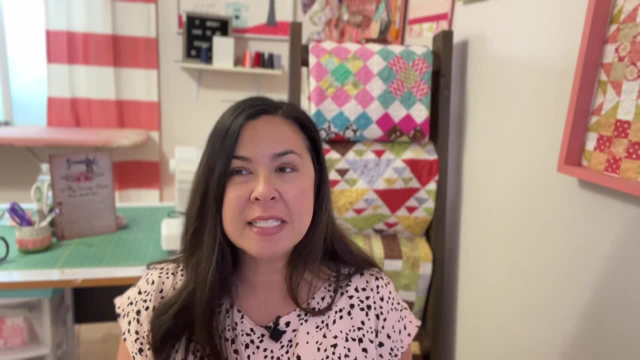 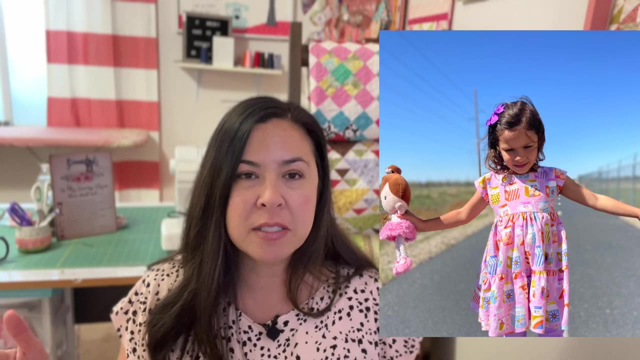 first one that I'm going to be talking to you about is the Lorne pattern by Little Lizard King And it's a pdf pattern and I love pdf patterns for kids because kids are smaller. When you print those pdf patterns you're not printing like a huge amount of paper. A lot of times it comes to 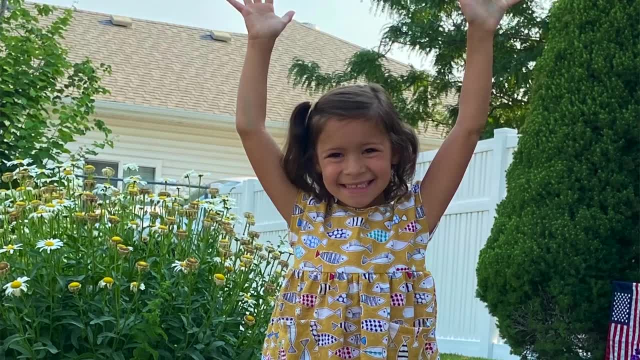 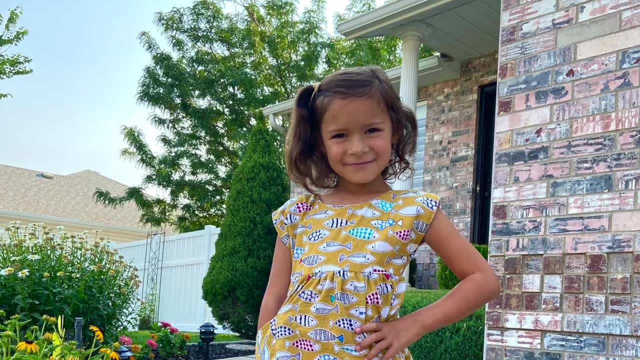 like two or three pieces of paper that you tape and then you're done, But they fit so much better than like McCall and Simplicity. The Lorne pattern is one of my favorite patterns and it's a pdf pattern for kids, As you can see in this picture right here. it doesn't have a set in sleeve and you can make. 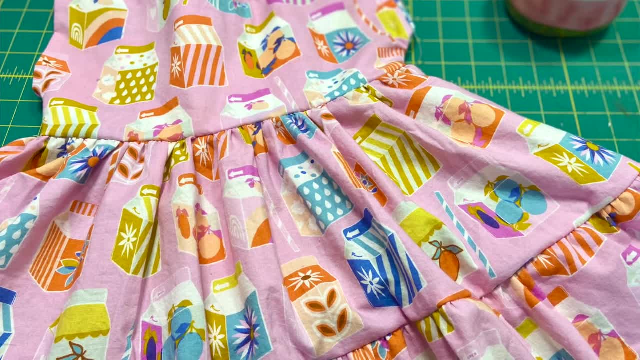 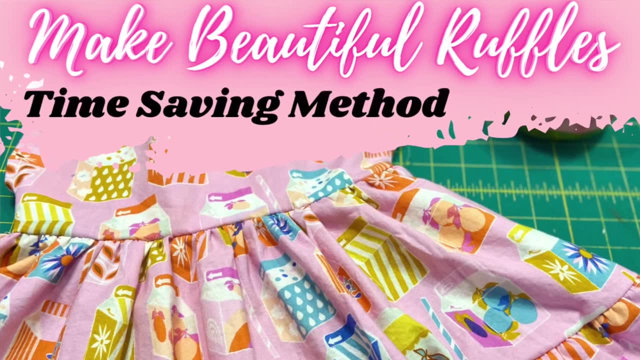 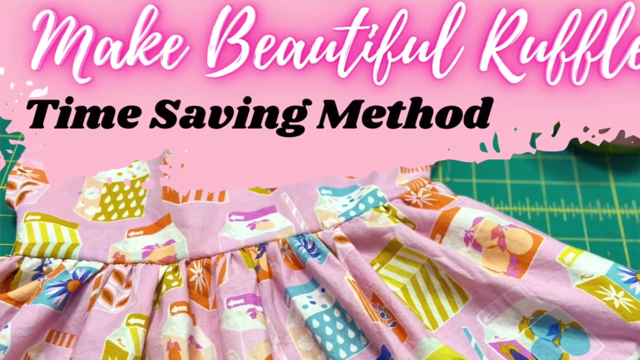 it with two tiers And it's just the front and the back, and then you add the bottom ruffle portion to it, And if you don't know how to gather fabric on your serger, you will want to check out this video right here. that will save you so much time in gathering fabric. You can make this Lorne pattern for kids for a variety of reasons, but I'm going to show you how to make the Lorne pattern. You can make it for kids. You can make it for your children. You can make the Lorne pattern for kids. You can make it for a family. You can make it for your kids. You can make. 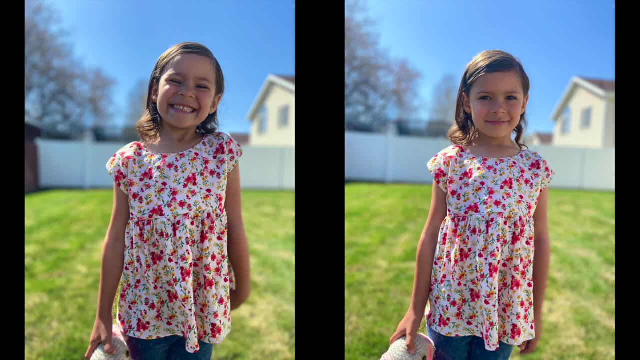 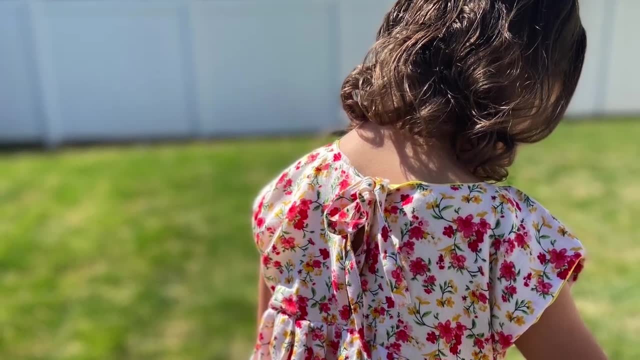 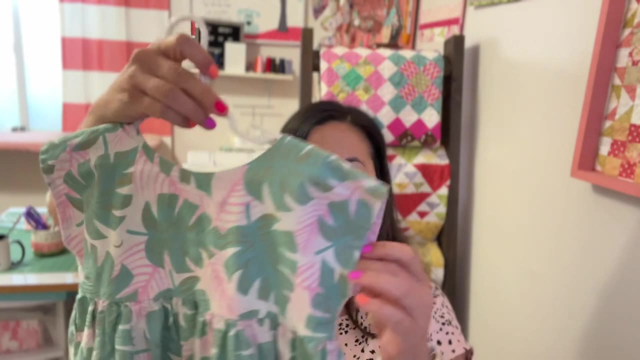 this Lorne dress into a dress, or- right here I have it where I made it- into this cute little tunic. but that one is actually perfect for school, and let me show you the back. so the back just has this tie right here and you, and the top is fully lined, and so it's just a fun, easy make. so this is. 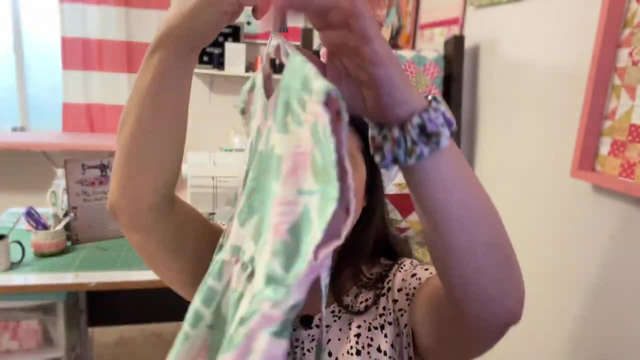 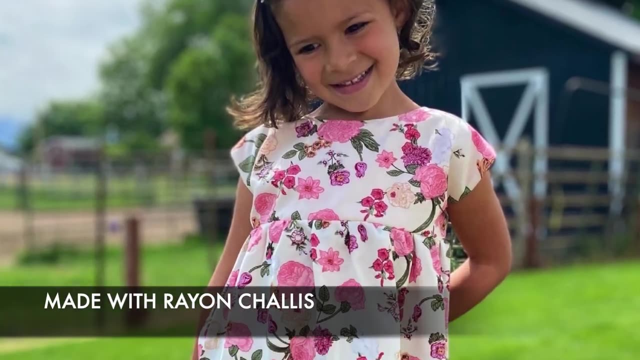 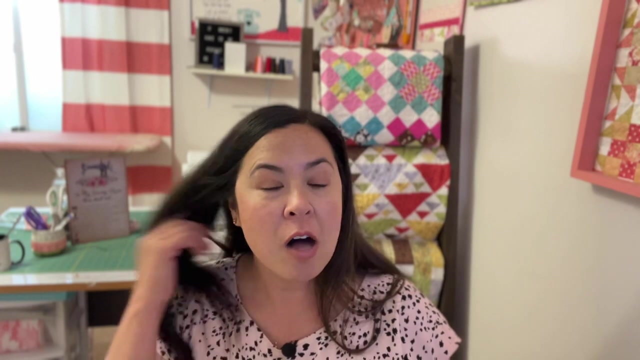 what the back looks like. and then you just do one tie right here and it looks like a tiny little cap sleeve. it's just one piece that you sew up together. also, you guys, I'm going to be leaving a link in the descriptions tab so that you can just 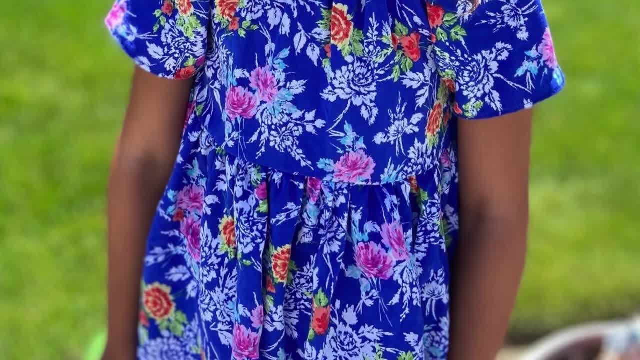 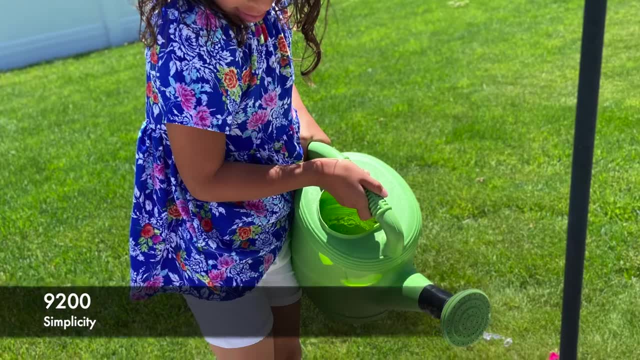 click on that if there is a certain pattern that you really love. the next one that I'm going to be talking about is simplicity 9200, and here is the pattern that I'm going to be talking about is simplicity 9200, and here is the. 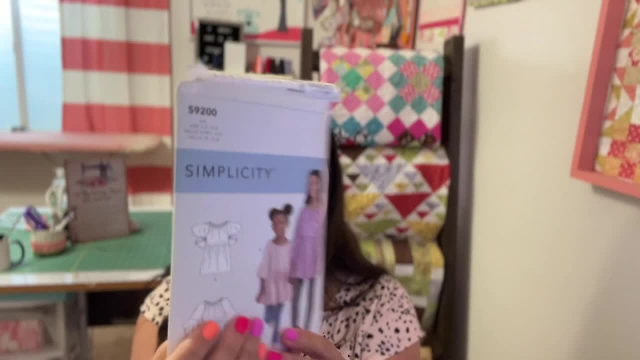 pattern that I'm going to be talking about is simplicity 9200. and here is the right here, and I'm going to show you even here's the line drawings. in the back it's supposed to be a tunic and I have a picture of my daughter right here. 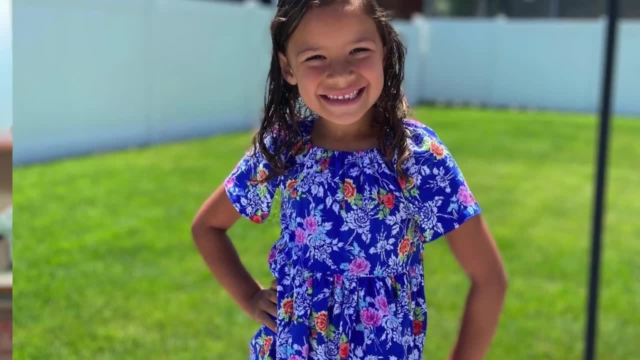 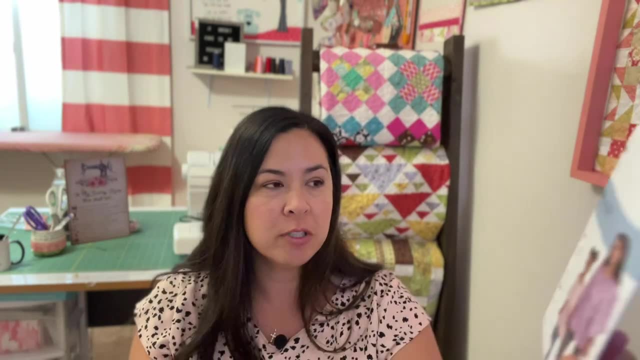 she's wearing it. I made hers in a view C but I didn't attach the ruffles. so you can do it, but I would. I love the ruffles. I would attach that on the next one. one thing that I want to warn you about the McCall's and simplicity patterns is: 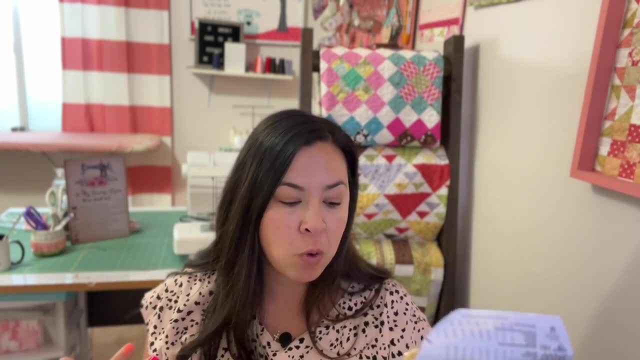 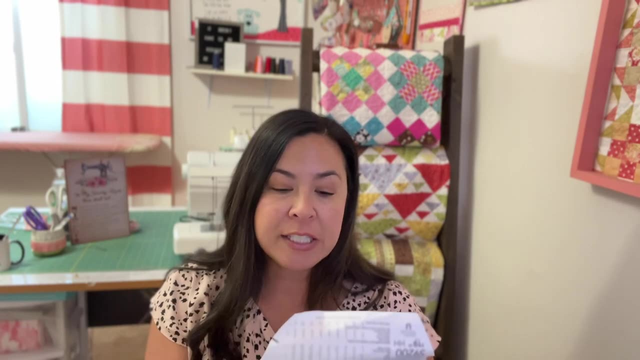 they're so huge, they have so much ease. and my little one, her chest is only 23 inches. let me read to you the description on here. this is size 3 up to a size 14. well, you want to look at the finished size measurement, because the 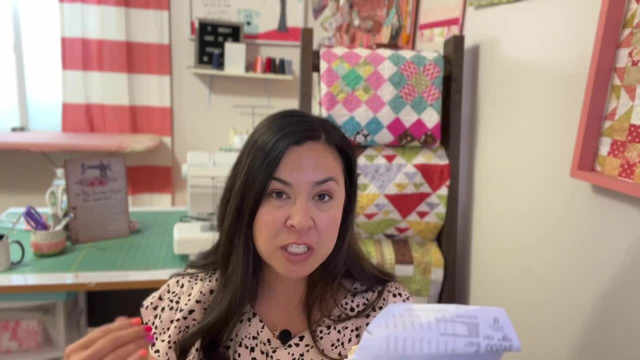 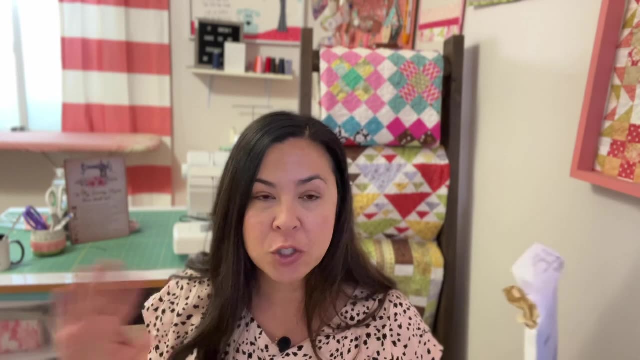 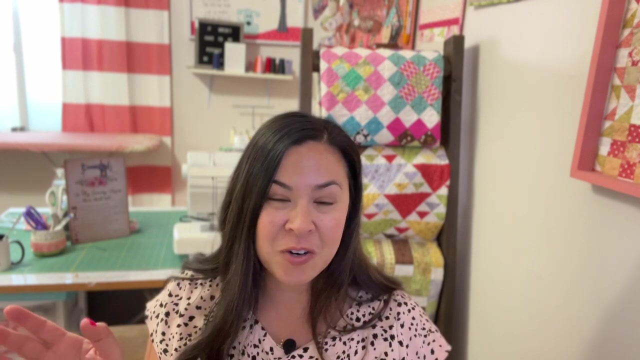 smallest on this one is 27 and a half inches. for the finished garment she's a 23. that would end up so huge on her that would have be so much extra fabric. so what I did is I took this and, and so even you know, let me emphasize- the size 3 is way too big on her and she. 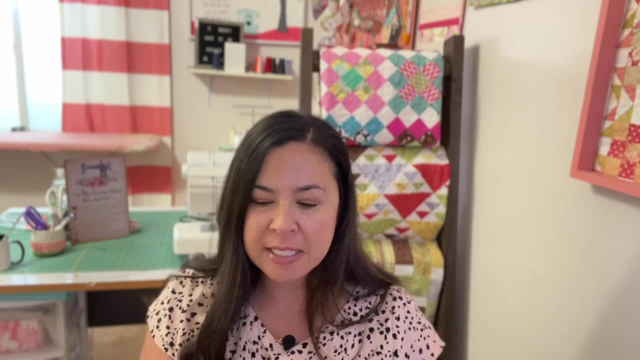 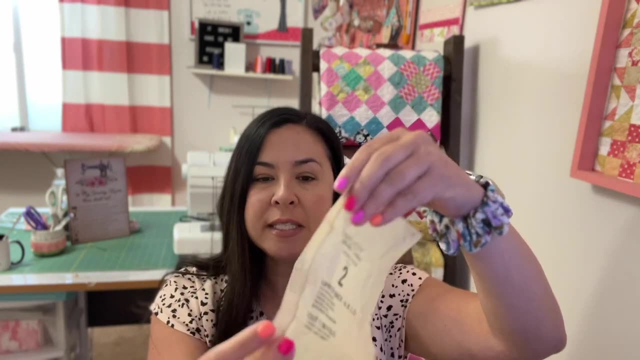 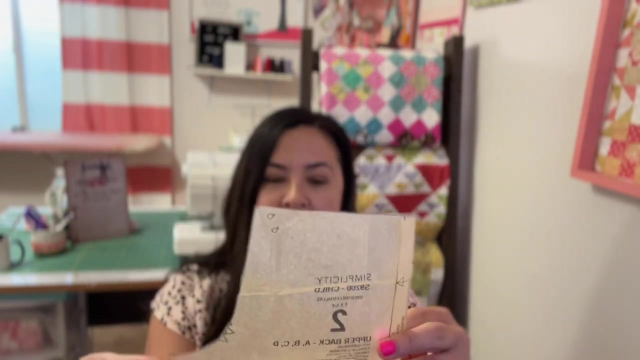 is a 7 year old now, so that's how much ease they have. what I did, though, is I folded it in here in the middle, so, basically, I took off. it would actually be an inch. it would be an inch that I took off of the inside, and then this: pattern. why this is it's\ downh explanation over the way W Buddha and you can go to get more of the rotten women printed style this pattern. why this works for her is because you're a 7 or 18. yes, she has over 25 other pieces of fabric and just that. 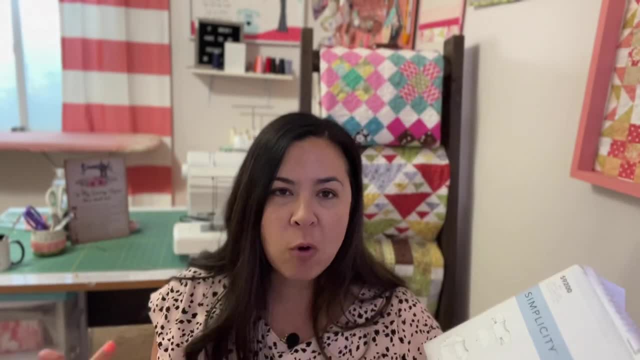 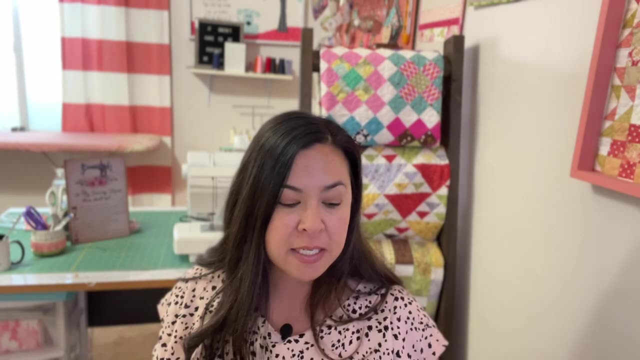 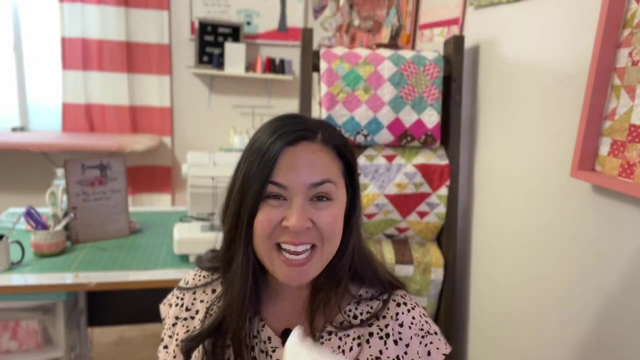 you've also has the. you have the elastic, so it's not a form-fitting dress, so I think I can get away with this. so I really do love this pattern and I recommend it because you could even lower it more to make it be a cute dress. this could be the cutest like first day of school dress that you 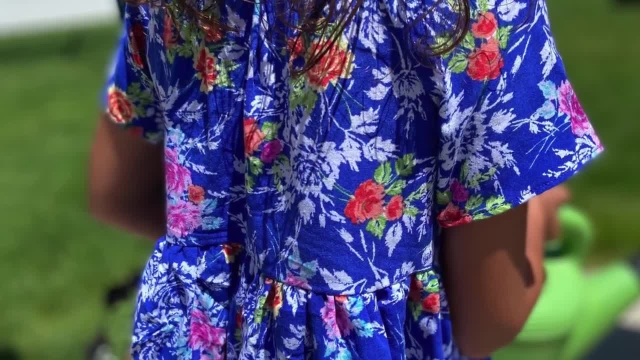 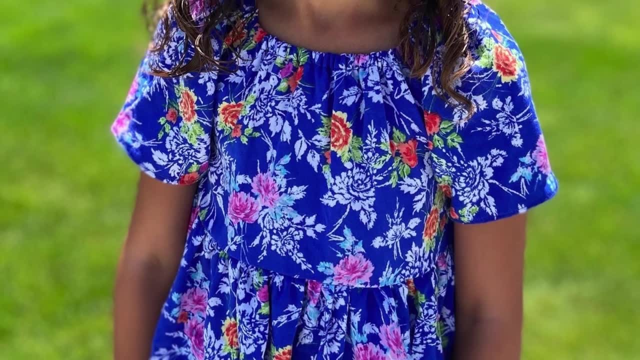 can make for your little one. I'm going to be making that one a lot more here soon. and what I did for the elastic: I just kind of wrapped it around her neck to determine the size that I wanted for that and on the sleeves I didn't alter the sleeves at all, I used the size three of the. 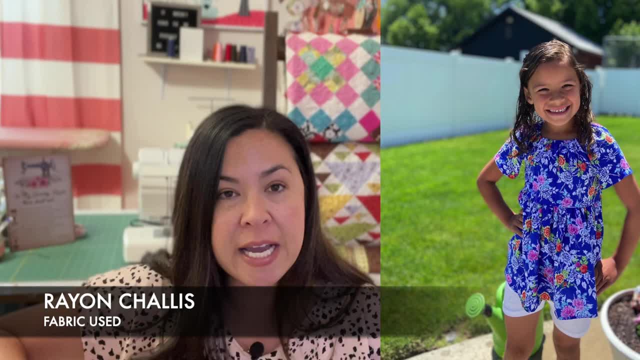 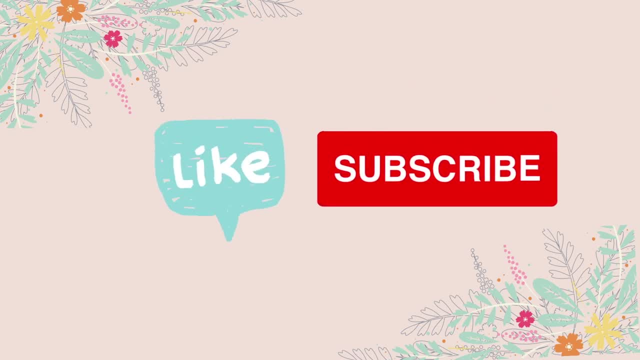 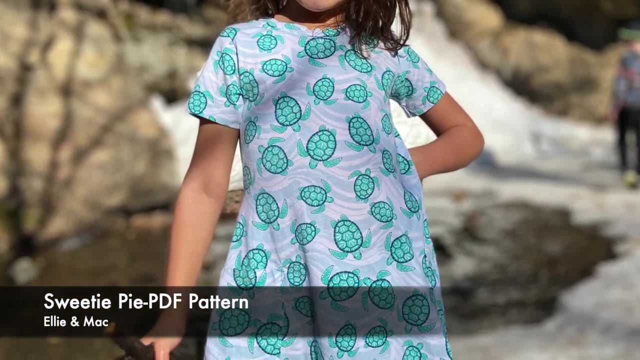 sleeves, and so all I did was make the chest area a little bit narrow so that it would fit her better. and also, if you are enjoying this video, make sure you hit the like and subscribe button, as it really does help support my channel. thank you. now the next pattern that I want to share with you. 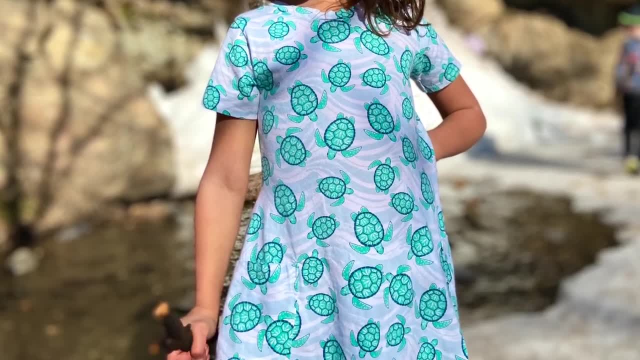 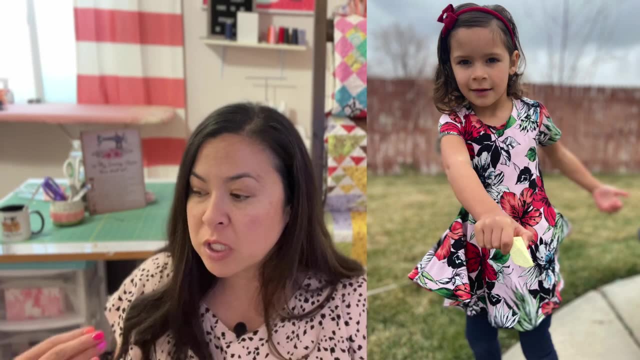 is a dress that I've been using for a long time, and it's a dress that I've been using for a long time is this sweetie pie pattern. this is by Ellie and Mac, and I have made this pattern several times and it is just a cute one-piece tunic dress, and so you sew the front up. there's. 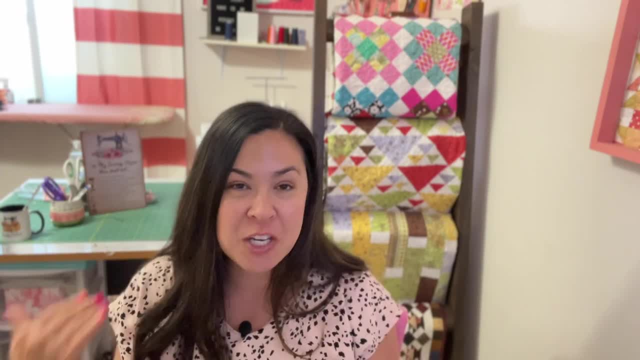 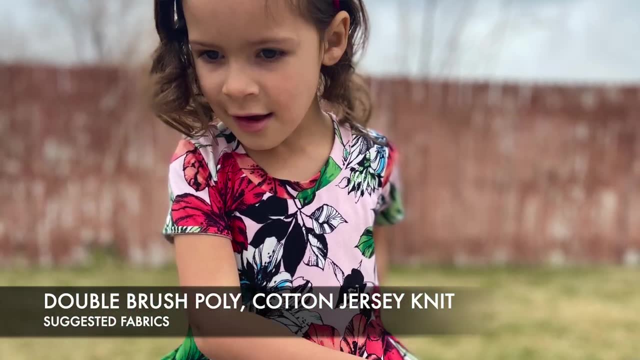 not even a separate bodice. you sew the front to the back and then you add the sleeves and this is just the perfect fit, and it's made out of cotton and or, I'm sorry, it's made out of knit. they gave you this Beispiel, L構icles Doesmcke 3DÓnesian watching video, and I'm going to show you. 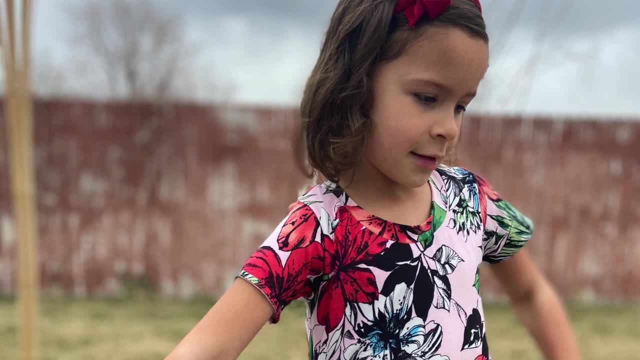 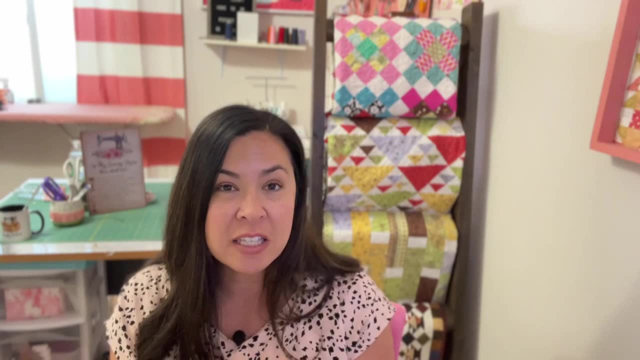 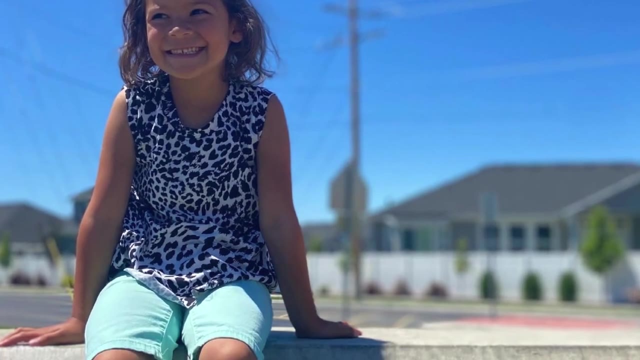 the neckband. it just all fits perfectly. i actually have a sewing video on the sweetie pie dress right there, if you want to click on that card, and i'm going to leave a link in the descriptions tab below where you can get this dress. you can make it into a tunic if you'd like this one. i left off the 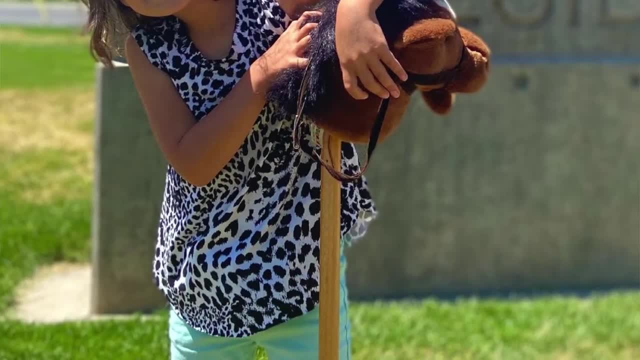 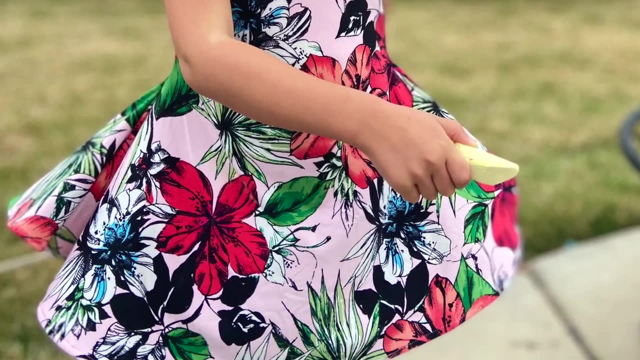 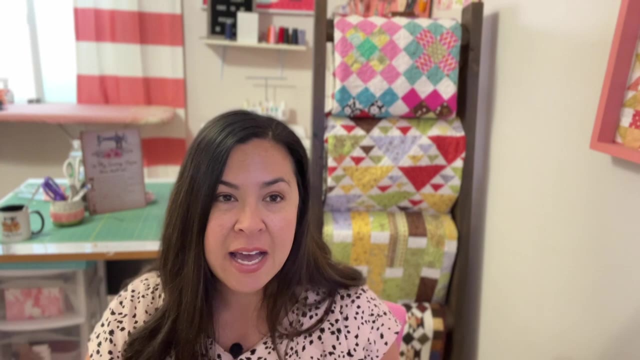 sleeve and i just added the neck bands. but really i've made this one so many times. it has a cute uh twirl to it where they would have a lot of fun twirling in it. but this one goes really cute with some ready to wear leggings and uh, or you can even just make a matching set in this one as well. okay. 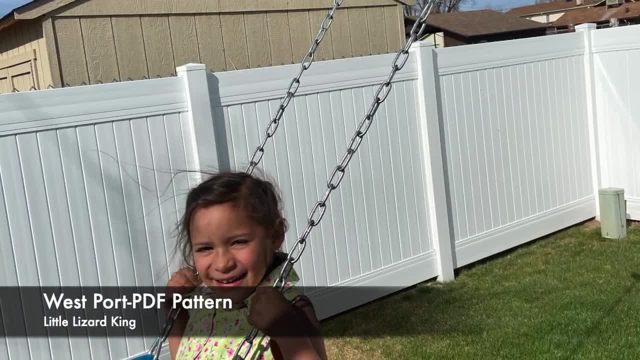 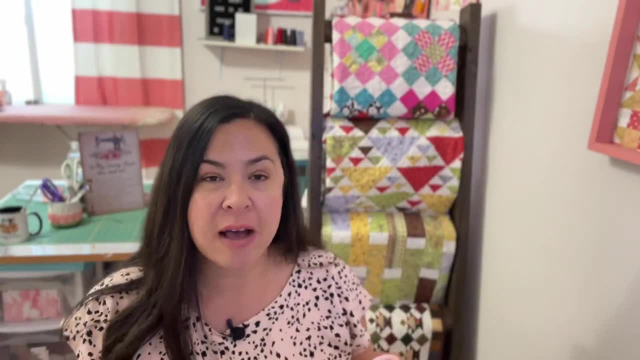 so this next one i want to show you is called it's the westport, and i love this one so much. they even have a boy's version. so if you have a son or a grandson that you want to sew for, you can sew them up. this br, this coolest button up. 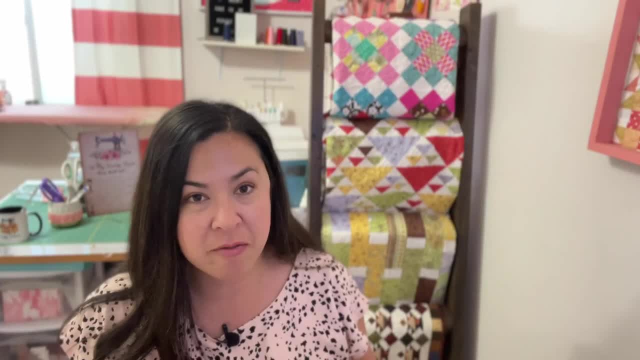 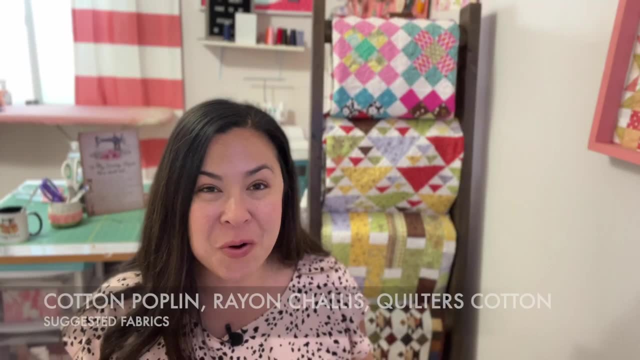 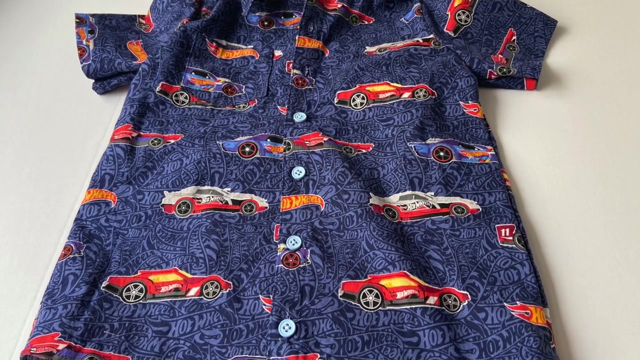 shirt and it's called the bayfield and that's a pdf pattern by little lizard king, and i can just imagine the cutest little boy going to school on his first day in just a shirt that he loves, like i made this one, um using a hot wheels pattern. 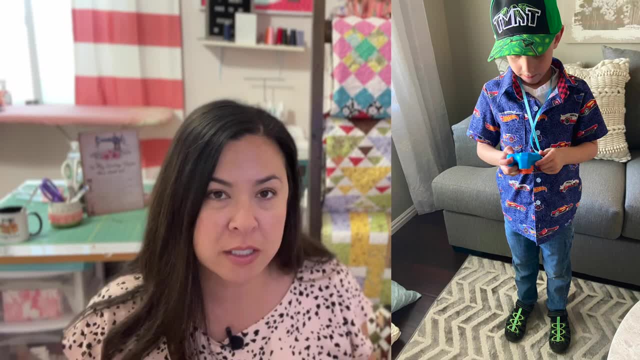 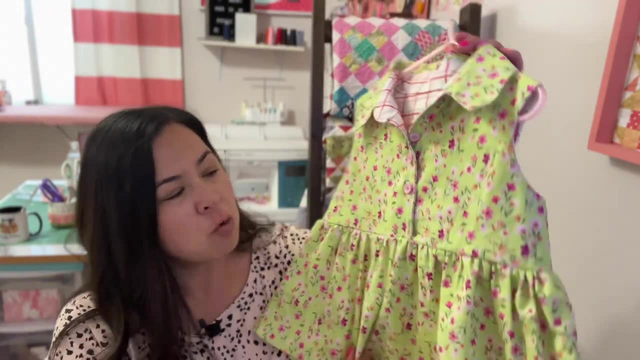 and this one is so cute. you make it with like a quilter's cotton, i think is the best pattern to make it with. so even this one i made it with the cutest quilter's cotton. i think this is like a right, and then you can make it with like a little. 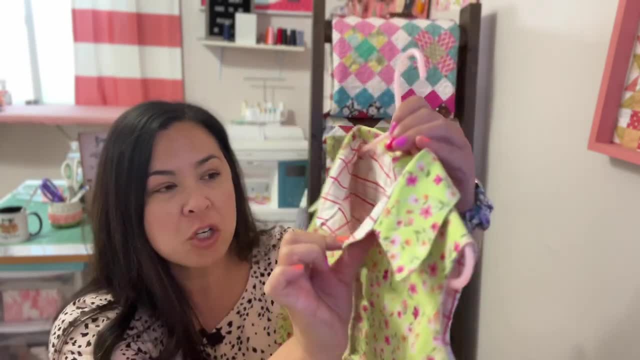 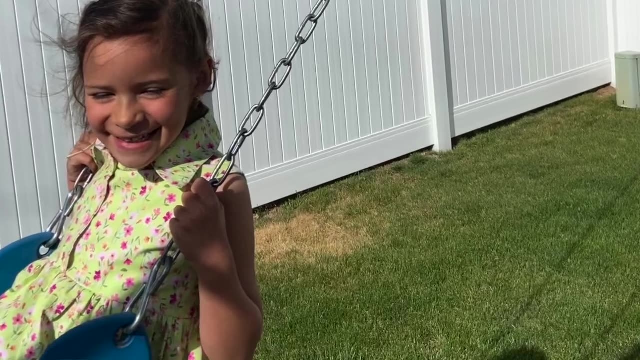 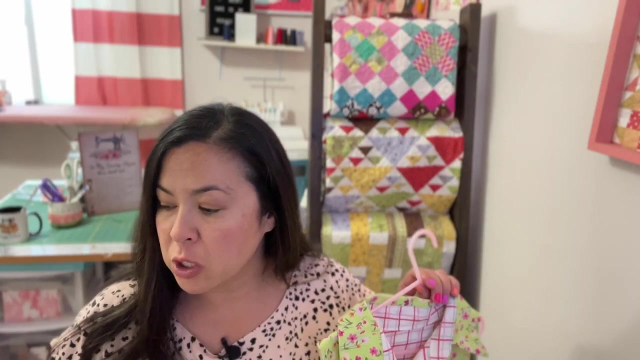 i just love the cute little buttons you can make. i just love the cute little collars and the contrasting neck band that you can put in here. this one on the girls: this is the westport and it's fully lined and you can make it into a tunic. i also made one into a dress, one thing that i recommend, if you. 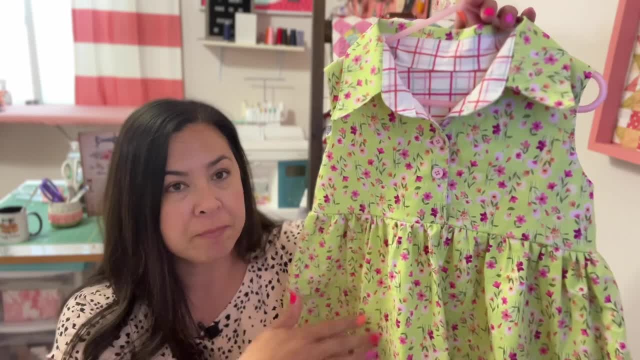 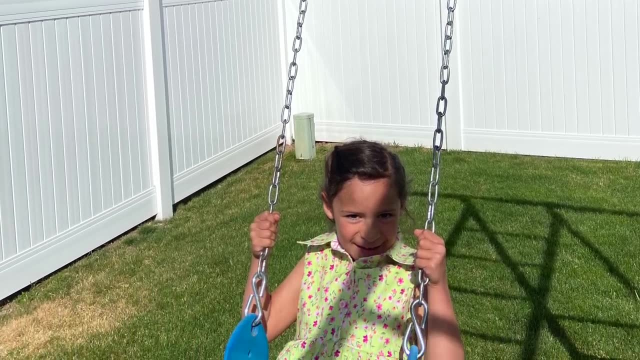 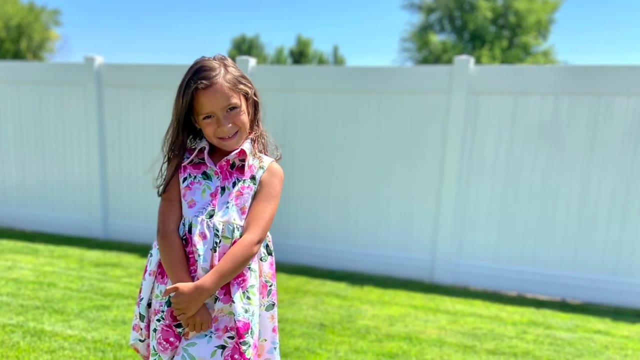 make it in a tunic, probably. i think it would be better to use like a poplin button or something like that for your dress, so that the top lays flatter more easier, it flows better. but when you're making the dress, that one, yeah, you can make it out of this quilter's cotton. 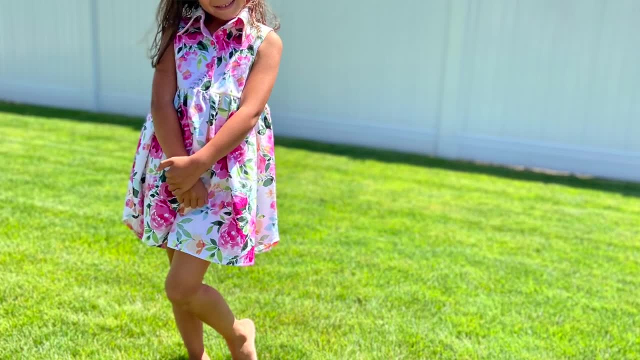 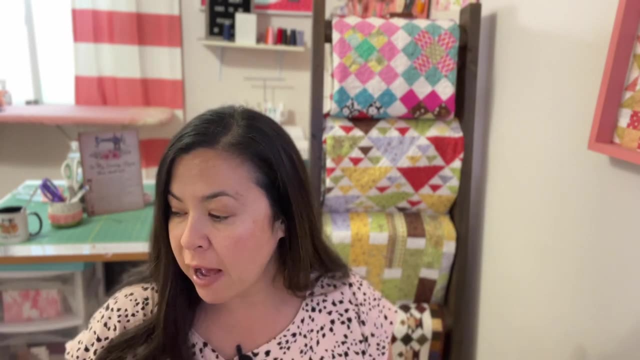 so let me show you a picture of this one. and this pattern also comes in the sleeveless version, and you can also make it in a long sleeve version. you can make it into a tunic or a dress, so you have a lot of options with that pattern as well. 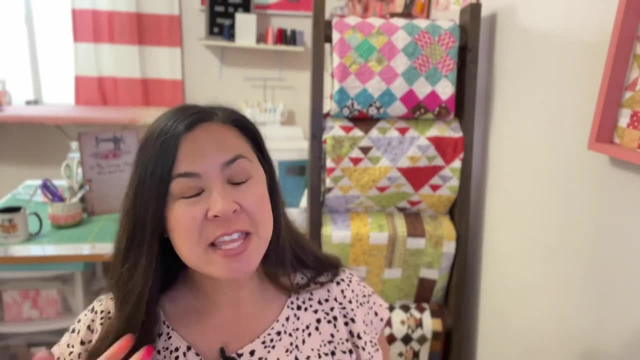 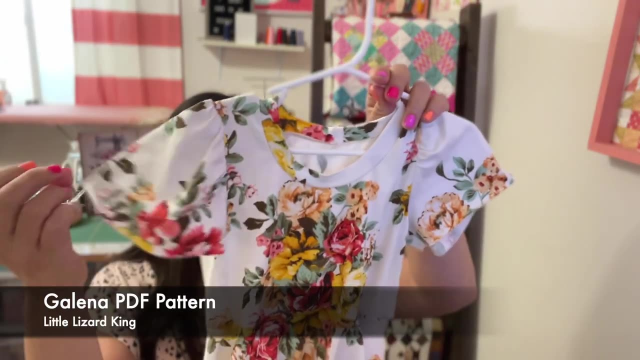 perfect for school. So I have another PDF pattern that I made from Little Lizard King as well, and it's called the Galena, and I've made it into a dress, I've made it into a tunic. I love these cute ruffled sleeves. It also comes with 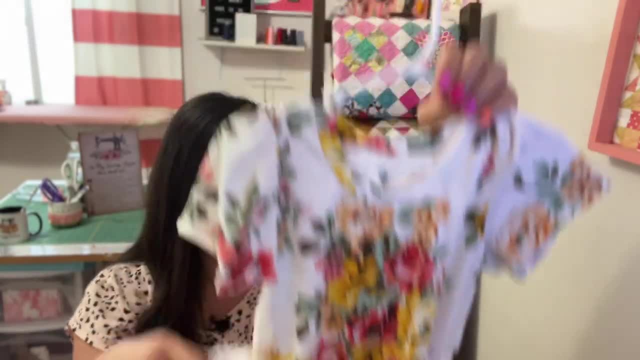 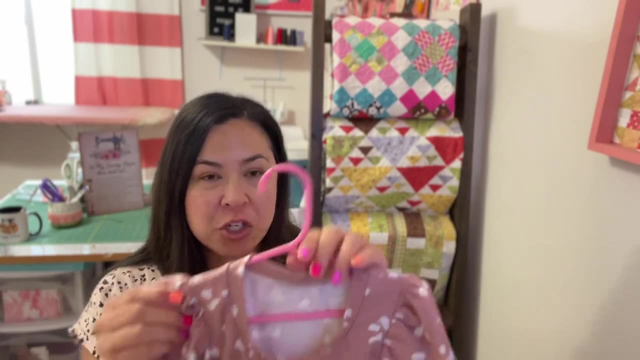 the neckband and it is separate. for the skirt. It's got like a cute little peplum top, So I have a few of them right here, but then also I've made it into just a plain shirt where I just extended the bodice. But look at how cute. 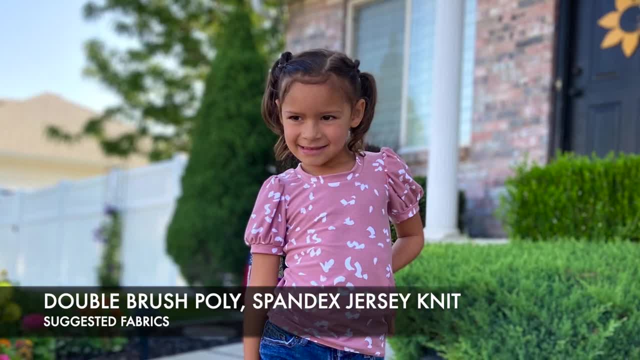 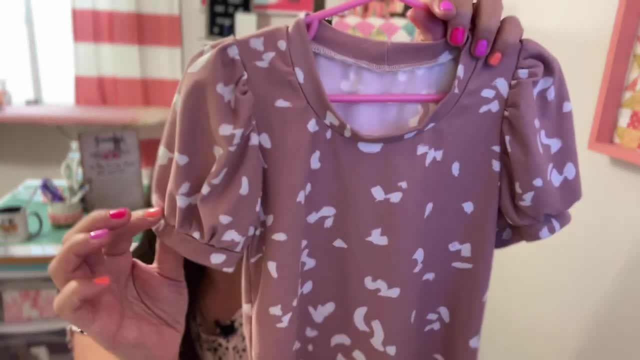 This one ideally is, you would make it with like a double brush poly. That's what I usually make mine with. And then look at how cute. Again, this is the Galena pattern, and they even come with these cute sleeve bands to sew up at the 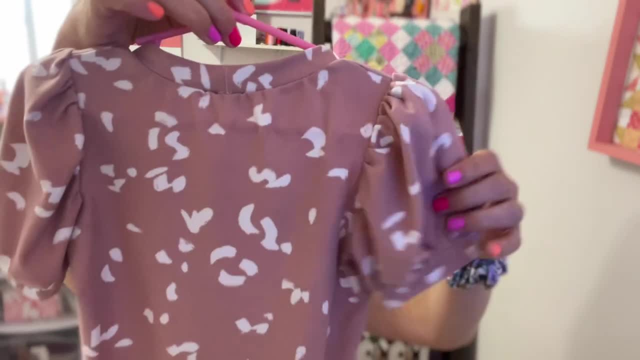 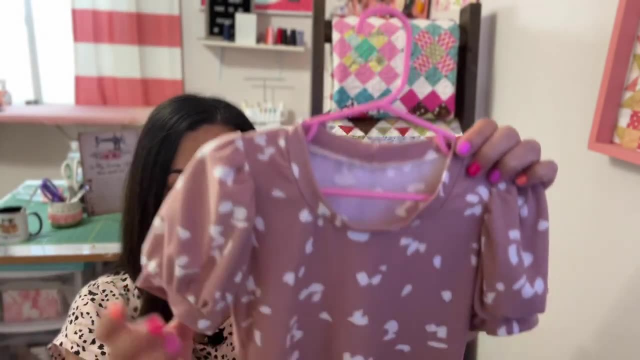 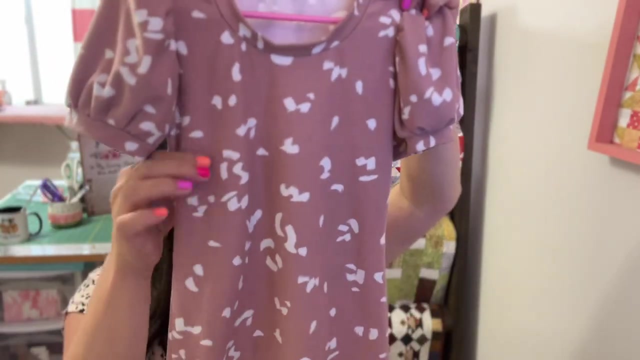 end of the cute little ruffle sleeve. This is one of my favorite shirts that I've made for her, So you could sew up a few of these to make for them for back-to-school, and so I think that one would be very cute as well. And again, you can make it into a little, into a shirt like this, or do like.